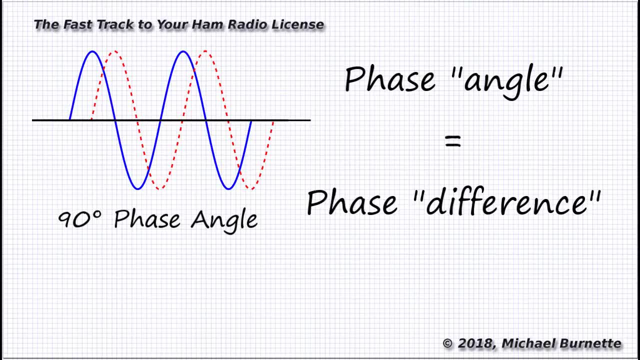 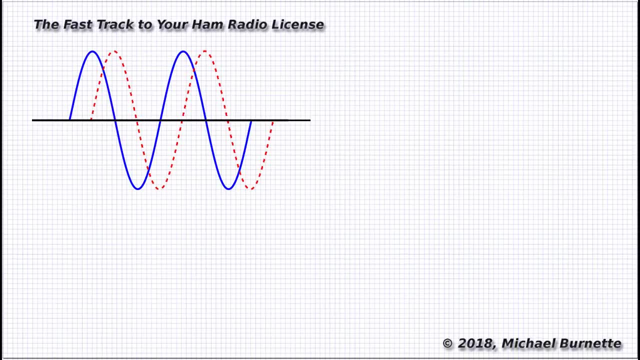 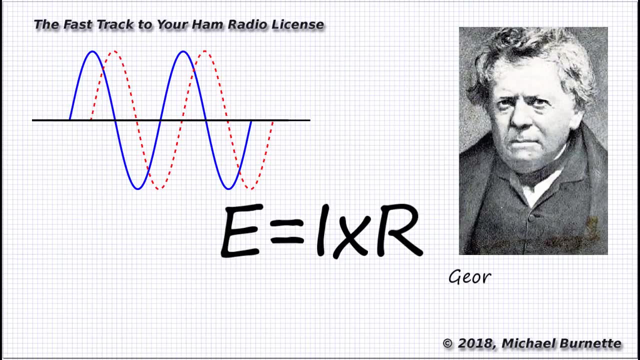 but those two are out of phase, and they're out of phase by 90 degrees. Now things get a little strange. When we learn DC electronics we learn that voltage and current always go together. Put a higher voltage on a circuit, the current instantly gets. 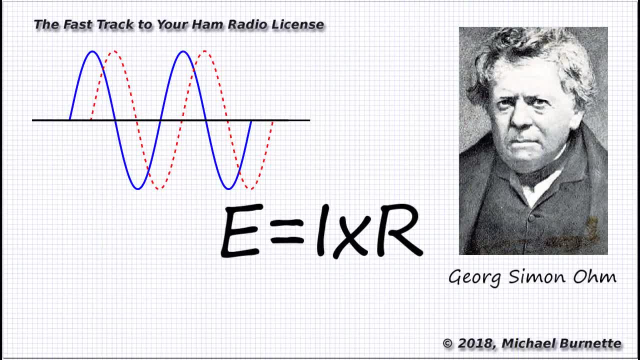 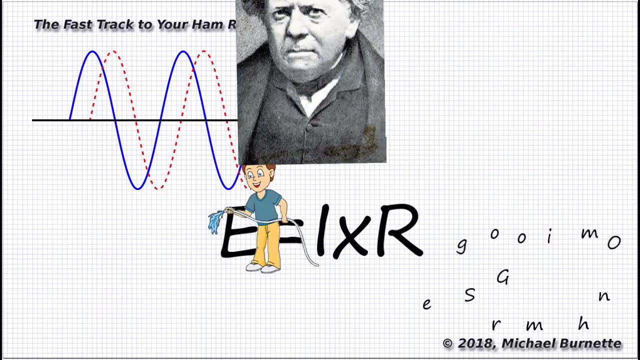 higher Because Ohm's law. I call it the garden hose model of electricity and I'm sure you've heard lots of garden hose related similes. as you've learned, DC electricity- The garden hose model- works great For DC AC circuits. make us kind of set aside that thinking In AC circuits. 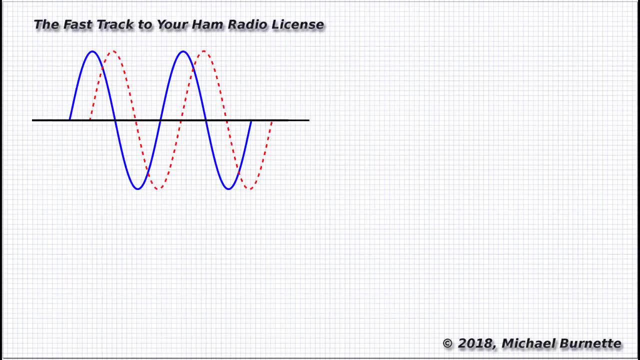 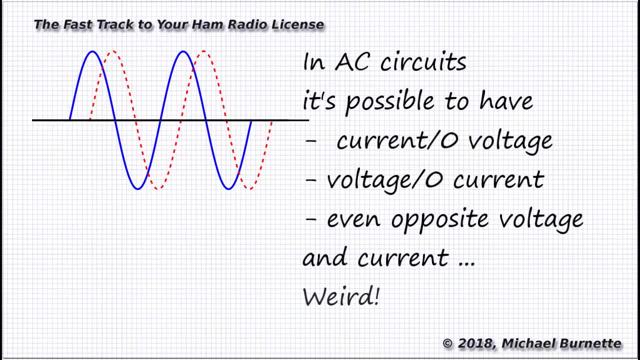 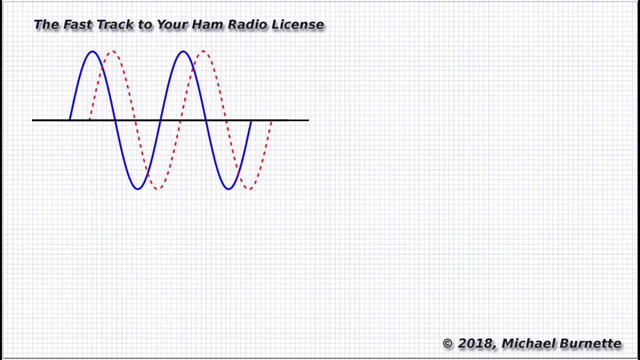 current and voltage can get out of phase. We can have spots where there's current with no voltage or voltage with no current. Current and voltage can be put out of phase by capacitors and inductors. So let's say in that illustration that the solid blue line represents voltage and the dashed red 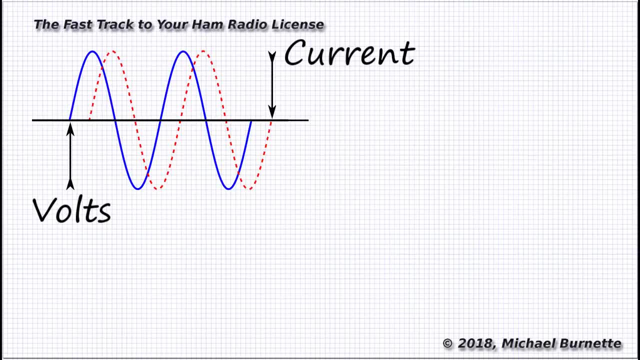 line represents the current. In that illustration, the voltage is leading the current by 90 degrees. In other words, the voltage is happening before the current Because, remember, that's time going across there on the x-axis and the stuff on the left happened before the stuff on the right. 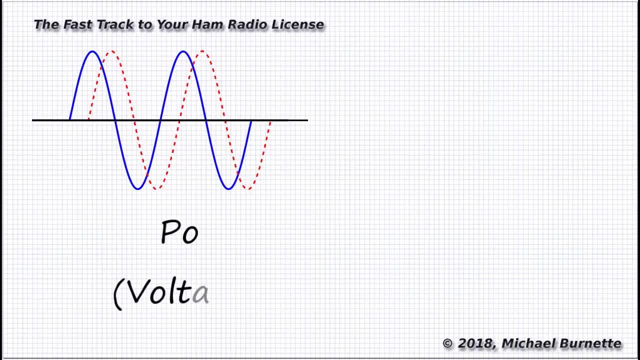 As you'll learn, that means we have a positive phase angle. When AC passes through an inductor, the current lags behind the voltage. Remember, as that voltage is headed up, those magnetic lines are going to be in the way of the current. So when AC passes through an inductor, 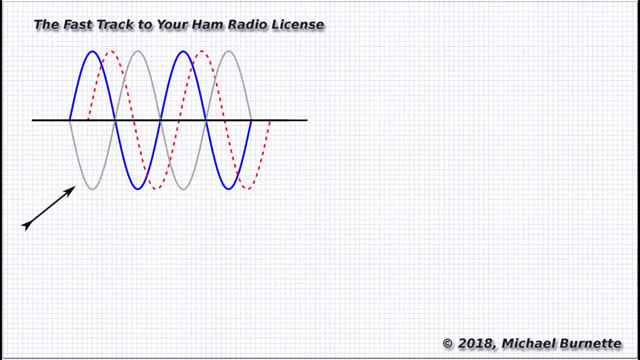 the lines of force are generating opposition to current flow as they grow. For simplicity's sake we'll say the inductor looks like an insulator to the current for those first 90 degrees of the cycle. Then the voltage peaks and it starts heading back toward zero and those magnetic lines of 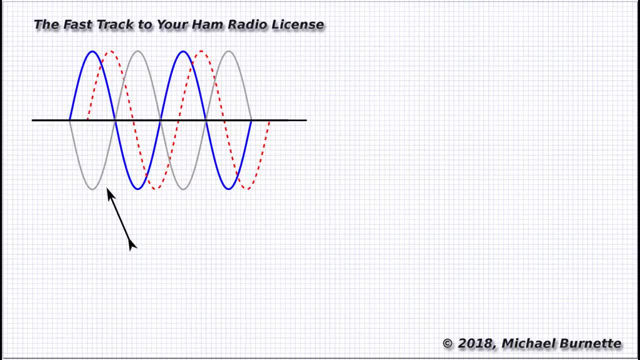 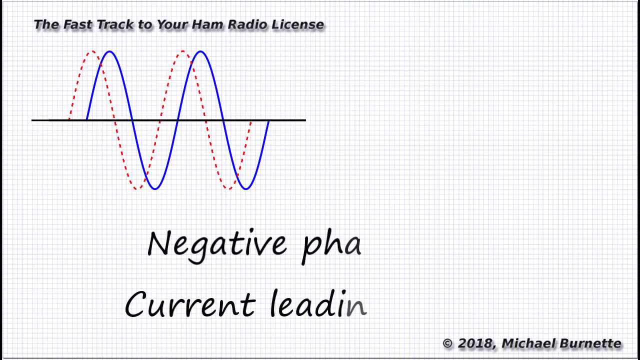 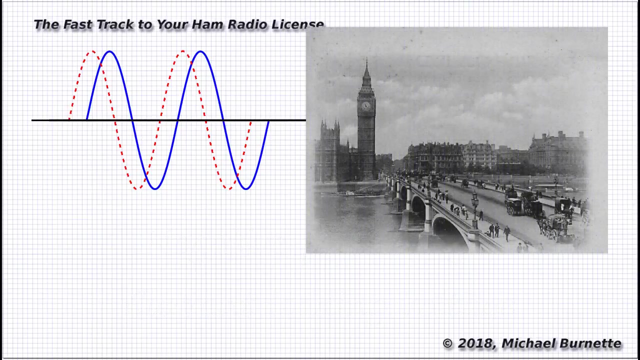 force start collapsing, creating current flow. The end result is: voltage leads current. Across a capacitor, the relationship is just the opposite: Across a capacitor, current leads voltage. Now there's a way to keep this straight in your head. The summer of 1885 in London, England, was dreadfully hot, Of course, in those days. 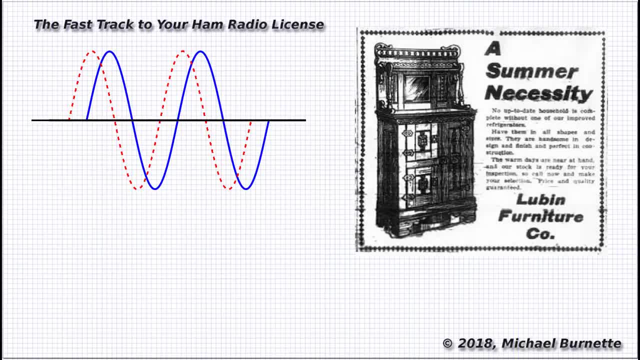 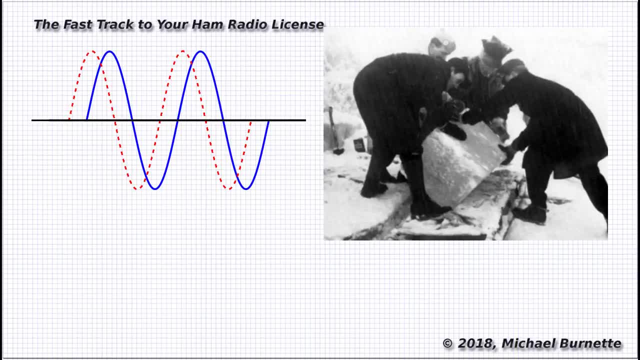 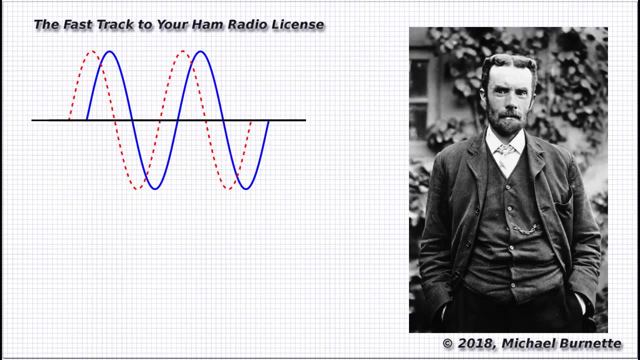 there were no refrigerators, but there were ice boxes and there were commercial ice services that would deliver big five-pound blocks of ice to homes to keep your food fresh. Now, during that summer, Oliver Heaviside was sweating away at his desk coming up with the equations that would lay the 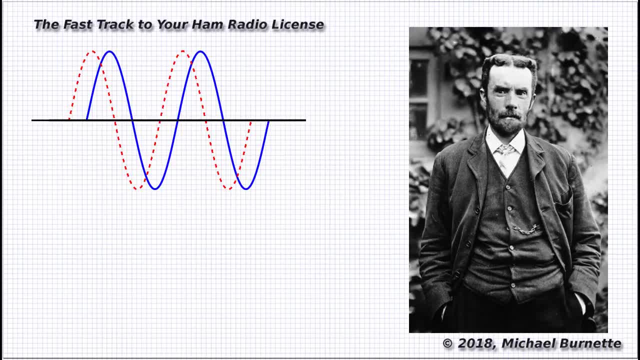 foundation for our understanding of reactances and impedances. Heaviside was absolutely brilliant, but he's all but forgotten these days. The man invented coaxial cable. he predicted the existence of the ionosphere. his telegrapher's equations made transatlantic telegraphy possible. 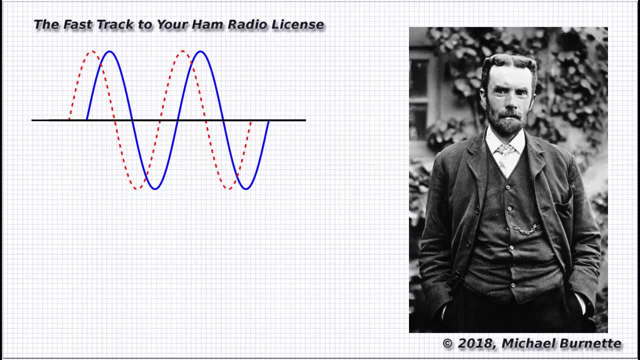 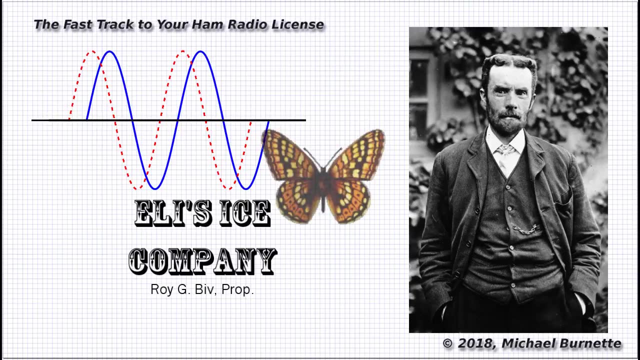 Well, every week Heaviside's meditations would be interrupted by his ice delivery from Eli's ice company. Heaviside was a notorious sourpuss and anything but a social butterfly. He was almost a recluse And Eli's deliveries always ended up in the middle of the night, and he was always. 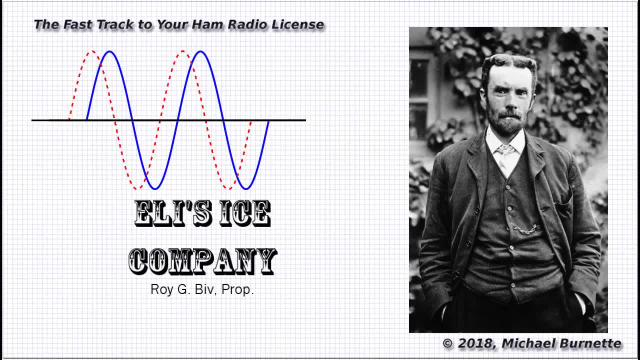 irritated. One day, though, he suddenly saw that Eli was unwittingly the perfect memory aid for the voltage and current relationships. Heaviside was discovering Gadzooks and a gad old chap. he cried. Voltage E leads current. I across an inductor L. 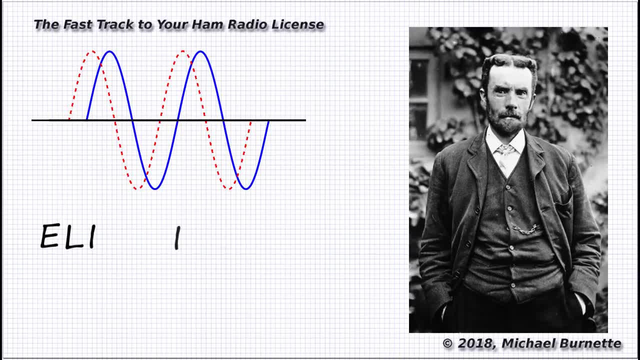 and current I leads voltage E across a capacitor C. It's E-li-the-ice-man. Oh, jolly good old bean. Ever since that fateful and, by the way, completely fictitious day, Ham's and other electronic students have used Eli the Iceman. 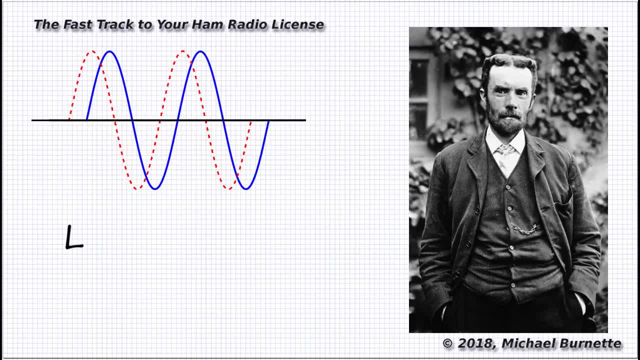 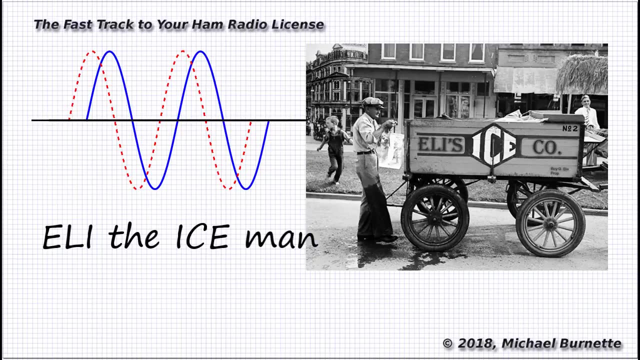 to remember that across an inductance, across an L E voltage, comes before I current E leads I. Across a capacitance, a C, I leads E, Eli the Iceman. And there he is right. there, It's an absolutely real picture. 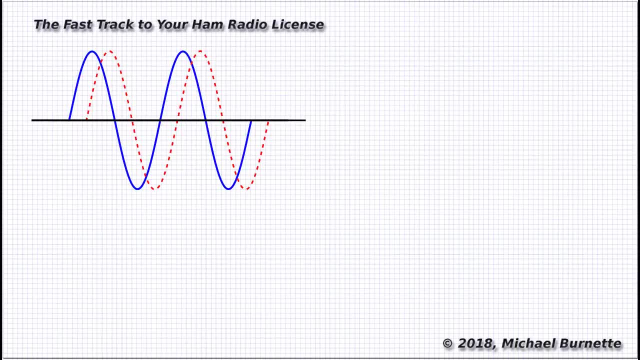 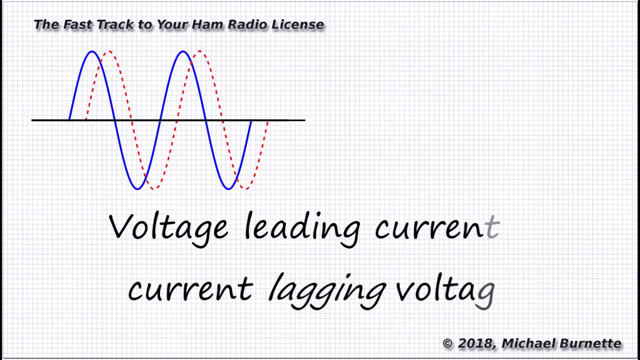 When we say the voltage is leading the current as it does across an inductance, we mean the voltage happens before the current. We could also describe that state of affairs as the current is lagging the voltage. They use both leading and lagging. 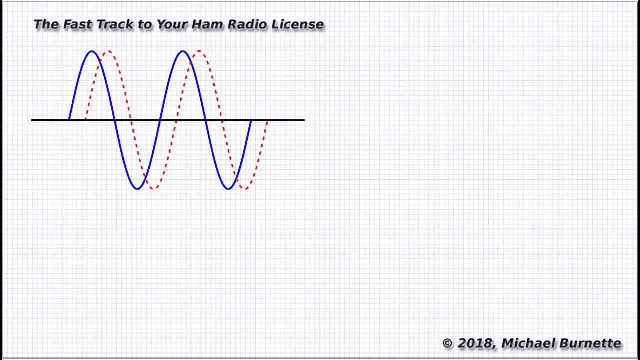 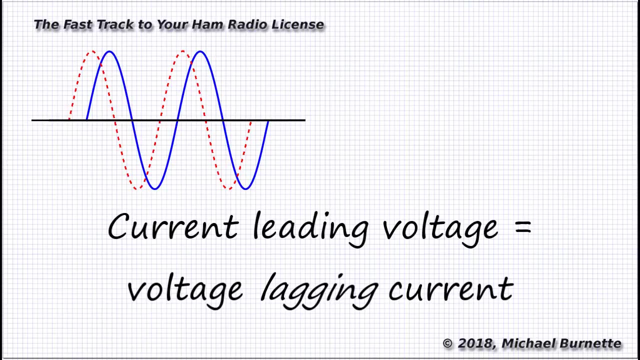 When we say the current is leading the voltage as it does across a capacitance, that means the current happens first, followed by the voltage. Of course we could also say the voltage is lagging the current. We're now fast approaching the topic of a series of questions. 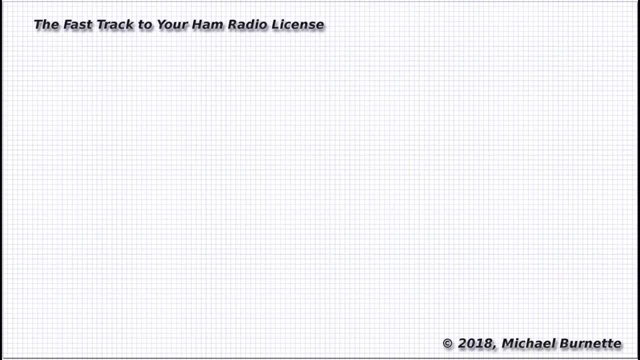 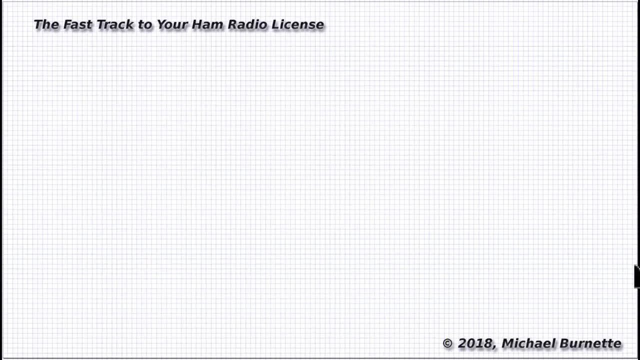 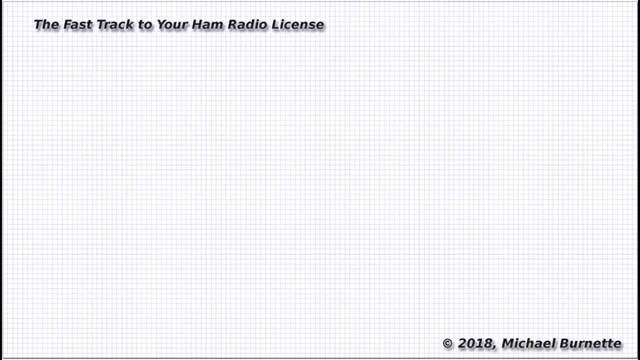 two questions out of fifty on the exam. I'll go through one of the three phase angle problems in the question bank, but if you have the Fast Track Extra course or our math workbook you probably already know there is what we might call an interesting and useful pattern to the answers. 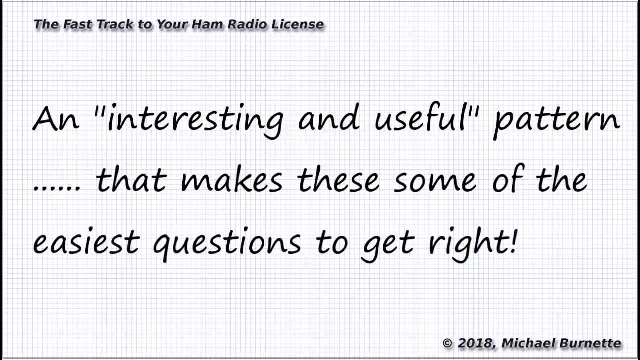 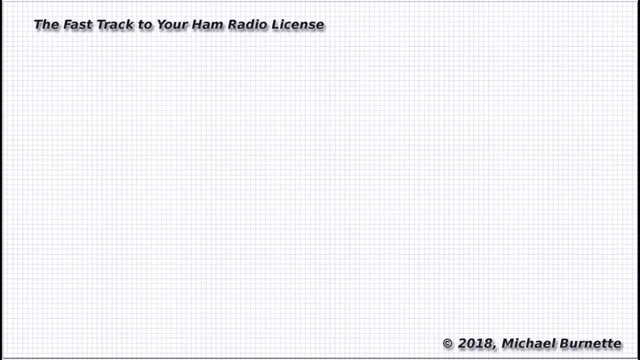 If you don't have those books, get a hold of the question pool and work out the answers and I think you'll see the subtle pattern. All right, here is one of the questions from the exam pool. It's question E5B07.. What is the phase angle between the voltage across? 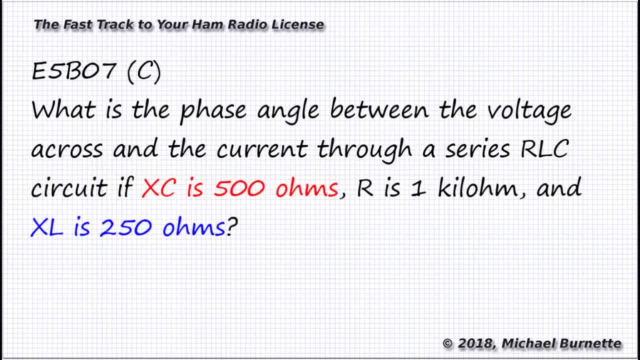 and the current through a series RLC circuit. if XC is 500 ohms, R is 1.0, and R is 1.0?. To calculate the phase angle of a series RLC circuit, we need the capacitive reactants. 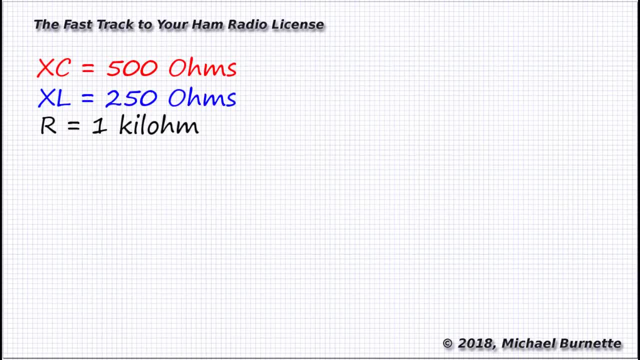 the inductive reactants and the resistance. They've given us all the values we need right there in the question. All we need to do is plug them into the right formula. Here's the right formula. It's phase angle equals tan negative 1.. That means the reciprocal of the tangent of XL minus XC over R. 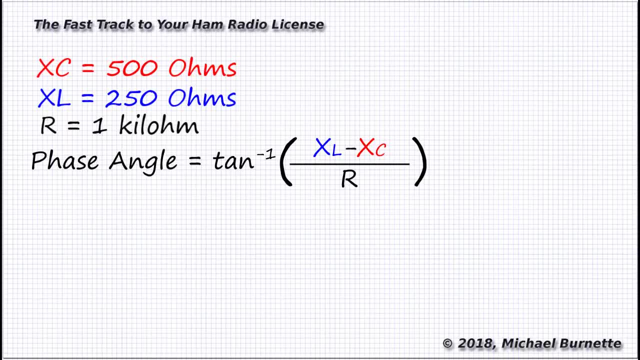 Now tangent negative 1,. the reciprocal of the tangent is also known as arctan or arctangent. Tangent is a trigonometry function. It's used in this case to calculate the angle formed by the adjacent and hypotenuse sides of a right triangle. 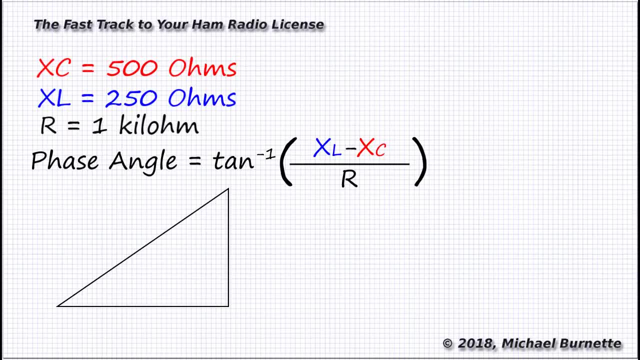 when the opposite and adjacent sides are known. These are just terms that are used in trigonometry to designate the various sides of a triangle. You have an adjacent side, an opposite side and then that long side which is the hypotenuse. Now impedance and phase angle problems can all 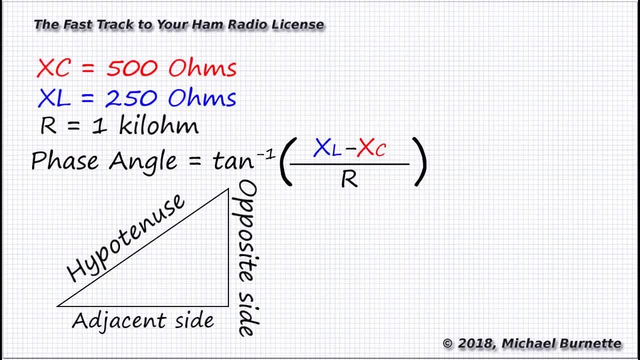 be diagrammed and solved as right triangles, with the resistance represented by that adjacent and opposite side. Consider that, running along the X-axis of a graph, The reactance represented by the opposite side and the impedance is the hypotenuse and the phase angle is represented by the angle. 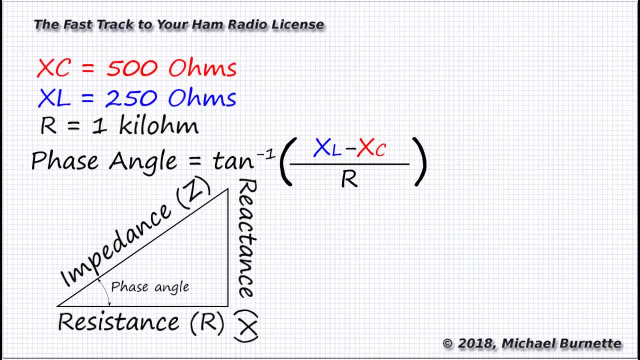 between the opposite side and the hypotenuse Isn't that cool. So that's what we're solving with this formula. The answer comes out in degrees Now that triangle can point to a right triangle, sort of one of two ways If we have more inductive reactants than we have. 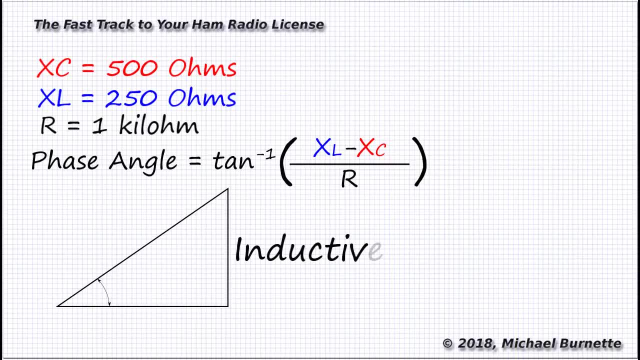 capacitive reactants, then the triangle is going to be upright, like this, and we'll have what's called a positive phase angle. If we have more capacitive reactants than we have inductive reactants, then the triangle gets turned upside down and now we have what we call a negative phase angle. So always. 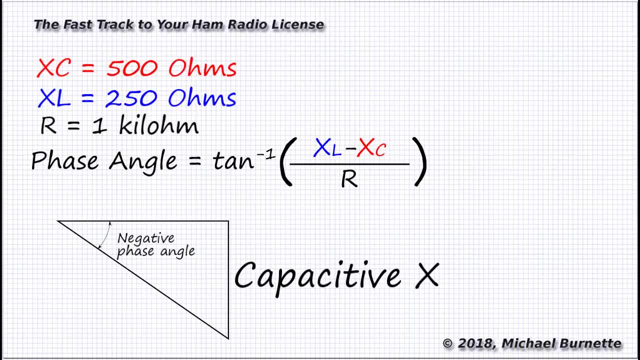 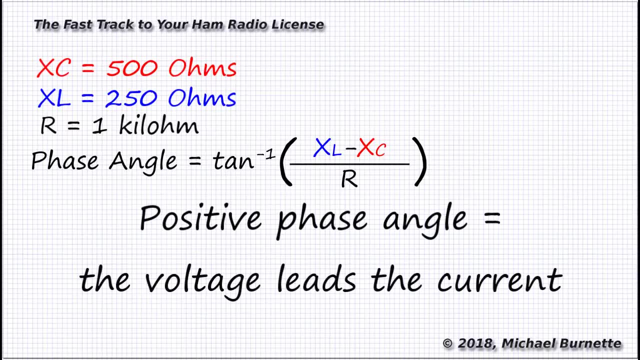 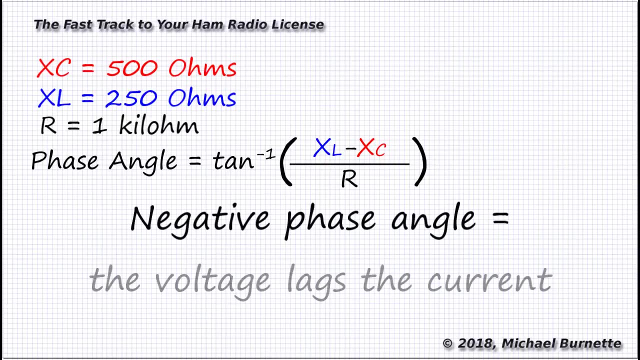 remember capacitive reactants is a negative value. That'll help you keep the formulas for this straight. If the degrees are a positive number, that means the voltage is leading the current. If the degrees are a negative number, that means the voltage is lagging the current. Think of it this way, Just consider that. 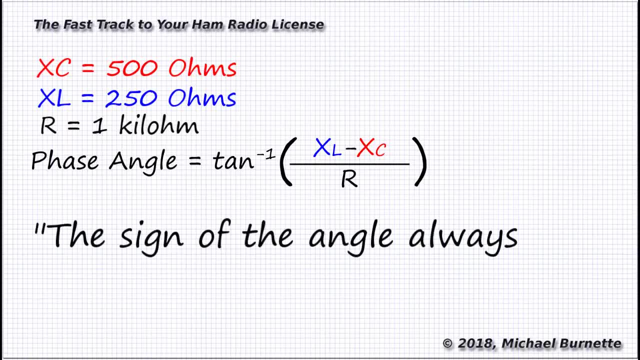 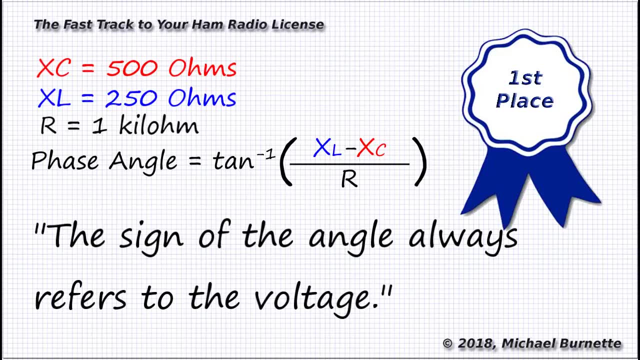 the sign of the angle always refers to voltage. If the sign is positive, the voltage is leading the current. If the sign is positive, the voltage is ahead of the current, It's winning the race. If the sign is negative, the voltage 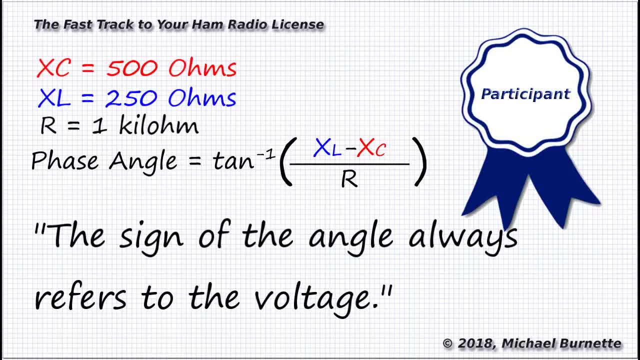 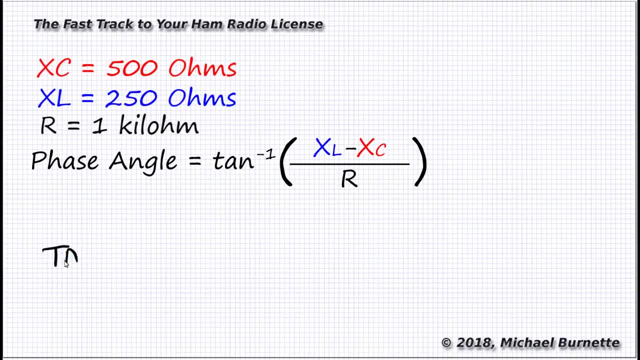 is behind the current, It's losing the race. So let's plug in our numbers. Phase angle equals tangent negative 1, or the arc tan tan minus 1, of 250,- that's the inductive reactants- minus 500,, that's the 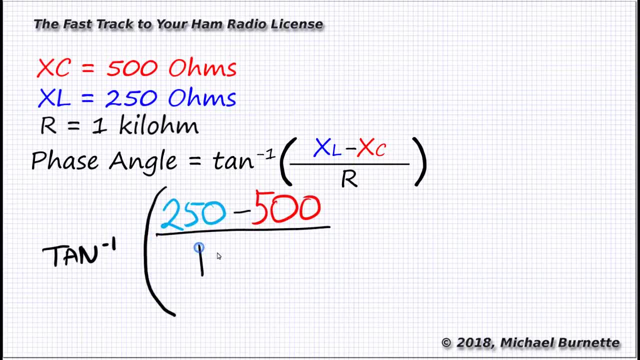 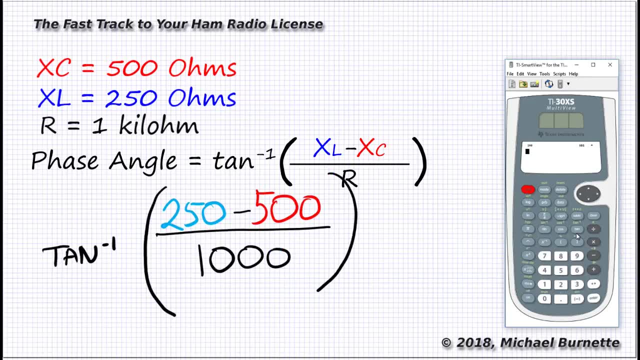 capacitive reactants over 1,000.. Let's plug it into the calculator. We'll go second key tan minus 1, then the numerator-denominator key 2, 5, 0, minus 5, 0, 0. We'll go down and do the denominator 1, 0, 0, 0, and we've got a. 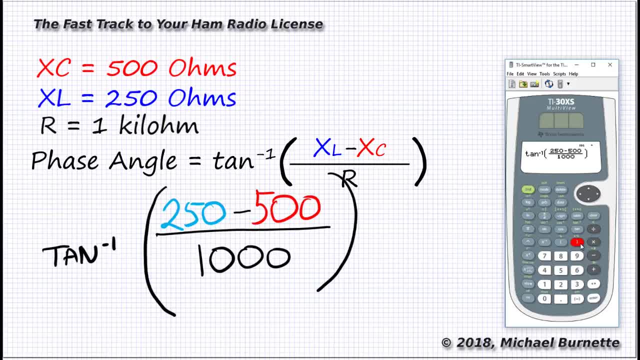 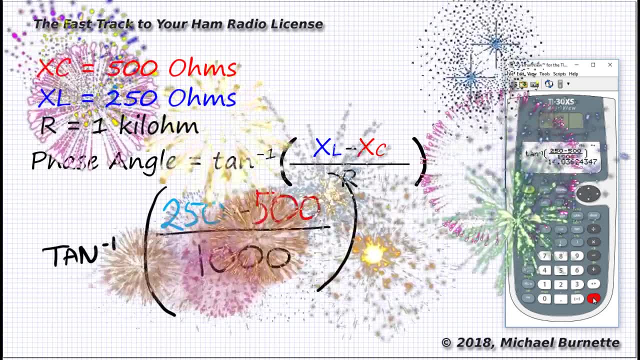 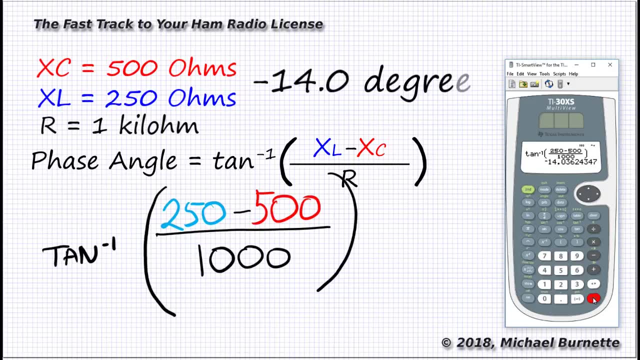 minus sign, We'll close off the parentheses. You notice that it automatically put the opening parentheses in there for you And we press enter And, ta-da, Minus 14.036. yadda, yadda, yadda, yadda, It's minus 14 degrees. The sign of the phase angle tells us where.